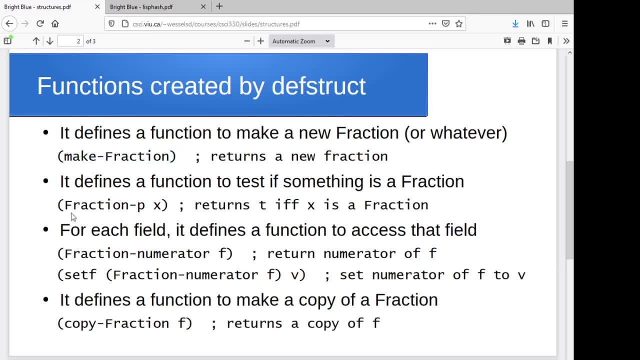 for the fields. It will create a function for you named fraction dash P or again whatever dash P to test true or false Is something a fraction for each of the fields. So this will create a fraction dash in that field name. So fraction dash numerator, for instance. 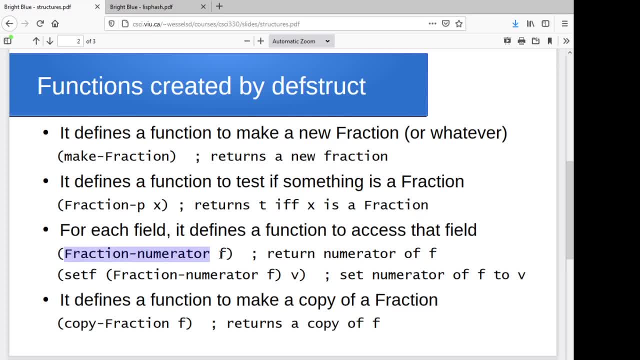 So just whatever your data type is, dash, whatever the field name is, And again this will return the value of that field for that fraction And you can use set F on it to change the value of that field. So set F and then the field look up and then the new value It. 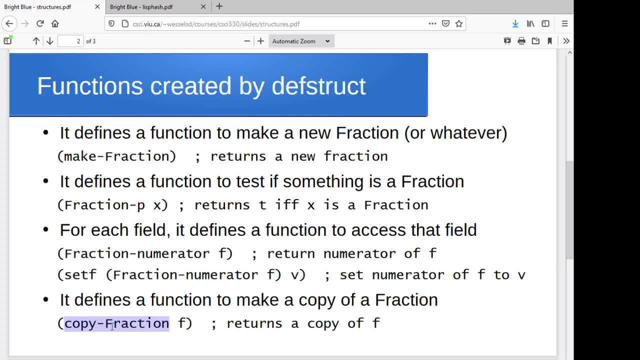 will actually give you a copy function as well. So copy dash fraction and then a new fraction to make a duplicate of the fraction and make, make a duplicate of whichever one you pass to it again. if you don't use copy fraction, then it's just doing a shallow copy, so you'll have. 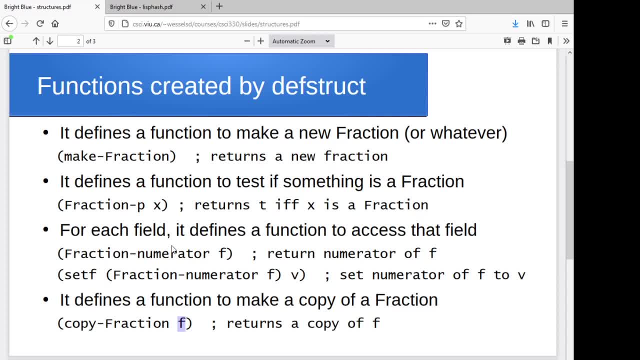 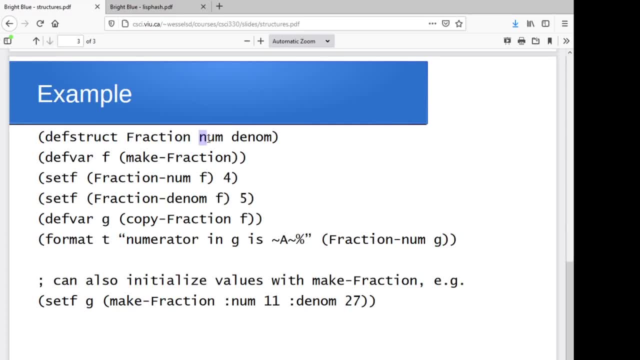 essentially two references to the same fraction. so do keep that in mind so we can go through. we'll play with this in just a quick example here. i'm going to be a little bit lazier with the field names, so i'm just going to call them num and denom. so i'm going to say: make a fraction. 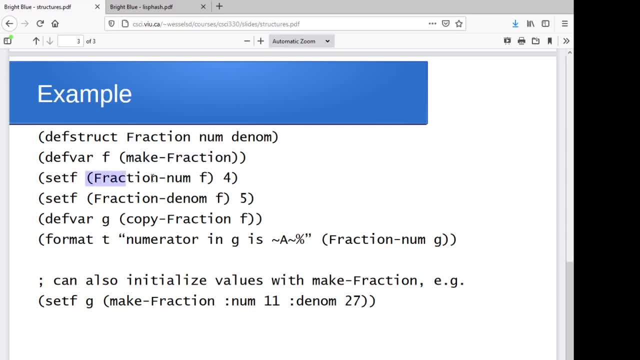 right and store it in f. set the numerator field to four, set the denominator field of f to five, make a duplicate of it and store it in g. so i'm just playing around here and let's print out the numerator field, for instance, of g, right, so we can go through and print that out. 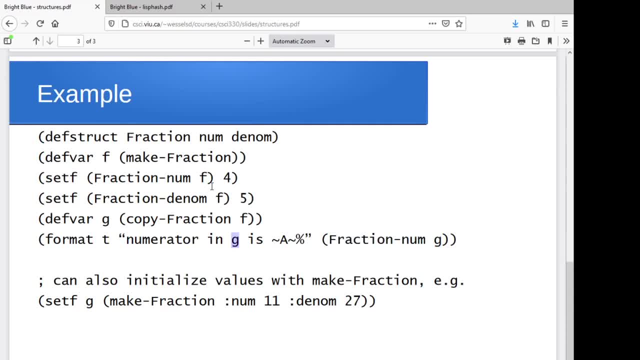 so it's pretty straightforward. you know, if you think about it with the tree data type that we looked at a couple of lectures back you. We had a list to represent tree nodes, where we had a list for the left subtree, a data value, and a list for the right subtree. 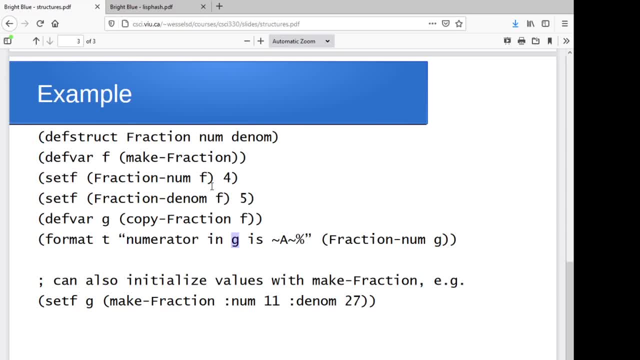 So here what we could do is say, well, let's give those named values, So let's set it up as a structure. So maybe we define a struct for a tree node and give it three fields: left subtree, data, right subtree, something like that. 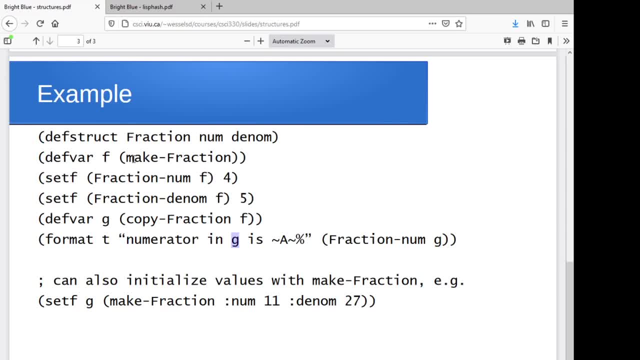 And then it's going to go through and give us things to say: okay, make a tree node, set the data value in a tree node, copy a tree node. So it would be quite useful. Now, one of the things I didn't mention with the makes is that you can actually initialize the value when you create the fraction or the tree node or the whatever it is. 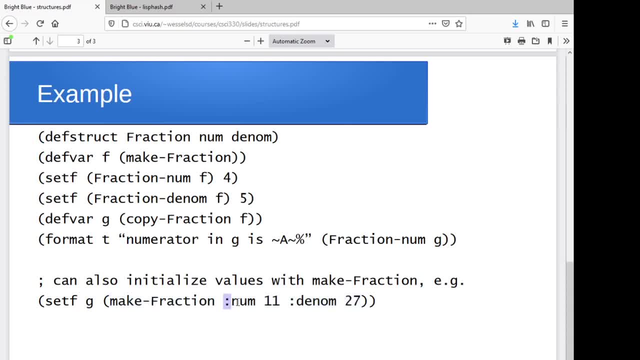 So it's: make fraction or make whatever, And then a colon and the field name And the initial value. So here I'm saying: create a fraction with 11 in the numerator and 27 in the denominator. So that is another possibility, All right. 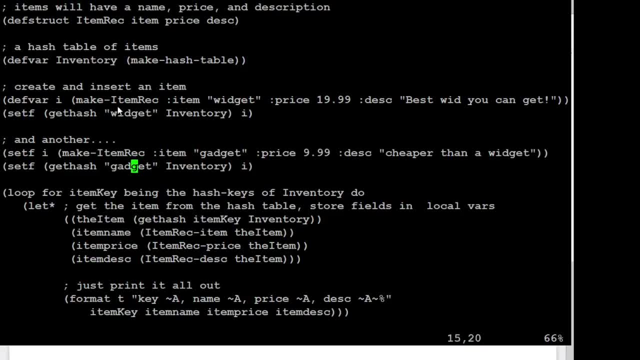 Just to give a quick playthrough on that. we'll go through And here we've got. we're defining a structure to represent items in some inventory. So an item record will have a name for an item, a price And a description for it. 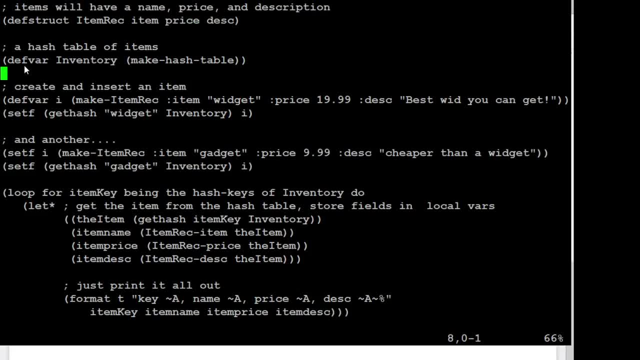 And what I'm going to do is create a hash table to create an inventory of all my items. So my inventory is going to be a hash table And, of course, it's going to be empty in the beginning. So what I'm going to keep doing is making an item and then adding it to the hash table. 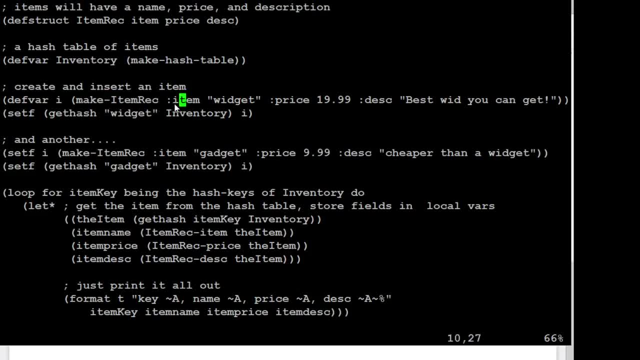 So I'm going to say: make an item, Give the name widget as the item name, Give the price as $19.99. And the description is the best widget you can get, Sorry. And then we'll add that to our inventory table. 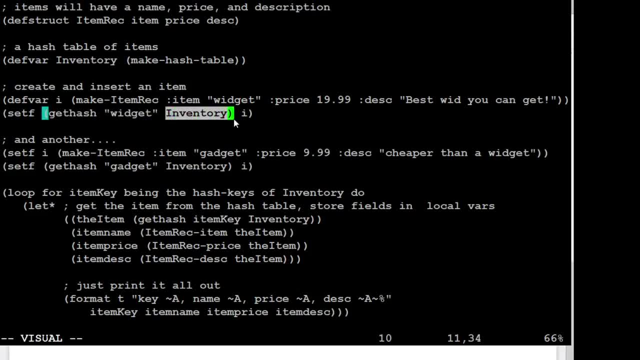 Right, So we're going to add under the key widget, we're going to add our item I to our inventory And so created one of these item recs and stored it in an inventory And we'll do the same thing. We'll do it again. 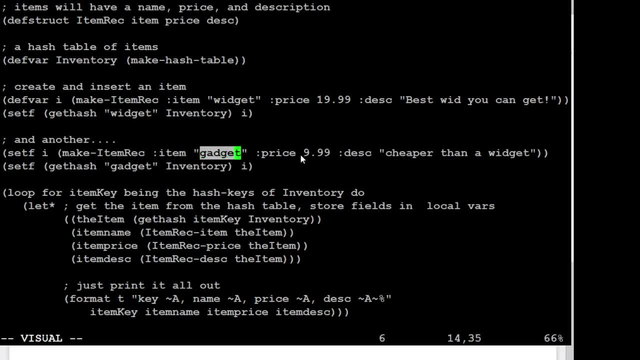 Let's do it, Only this time we'll give the item name gadget And we'll give a price of $9.99.. And we'll give a different description And then, And then we'll store that under the key gadget in our inventory. 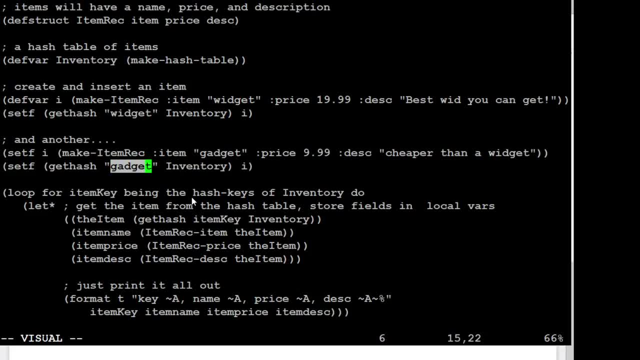 And so we can go through and just create a bunch of these things And then, just as another example of playing with loops and hash tables, we'll do that loop for item key. So item key is going to be the variable I'm using to iterate through.